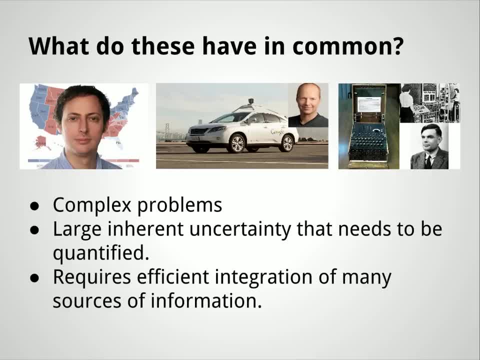 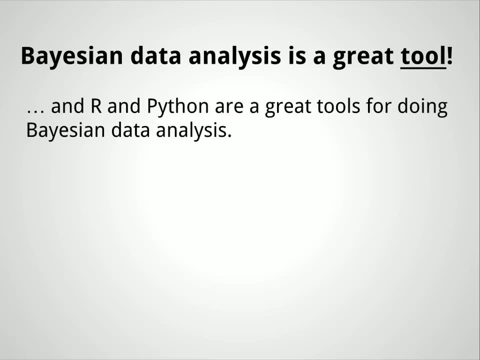 on complex problems Where there was a large inherent uncertainty that needed to be quantified and required efficient integration of many sources of information. And they all used Bayesian data analysis- And that's because Bayesian data analysis is a great tool- And R and Python. 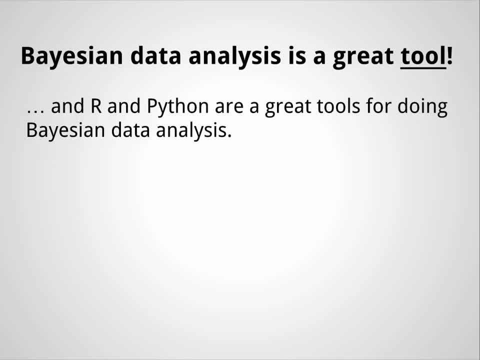 are great tools for doing Bayesian data analysis, But if you Google Bayesian, there's a good chance you won't find articles about how this tool could be used. Instead, you might get philosophy. You'll find articles discussing whether statistics should be subjective or objective, whatever that means, or whether statisticians should adhere to frequentism. 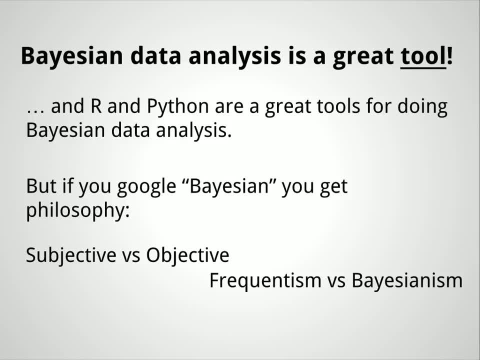 or Bayesianism, as if there were different religions within statistics, And you will find heated arguments about whether one should use or should not use subjective probabilities rather than p-values, And in this tutorial I won't talk about any of this. I will just talk about Bayesian. 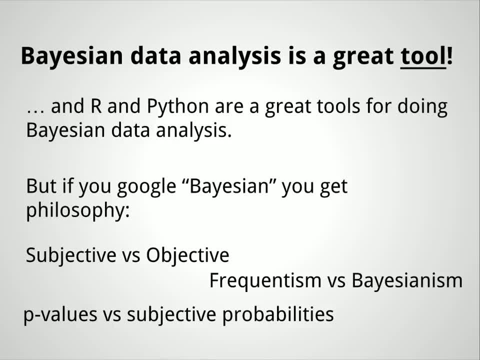 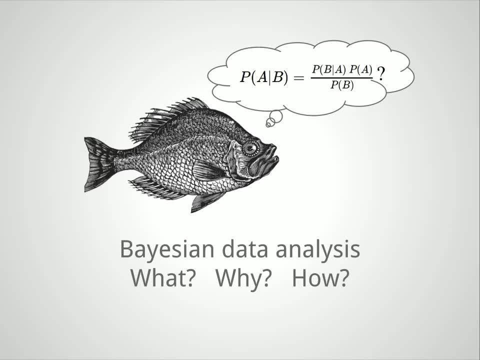 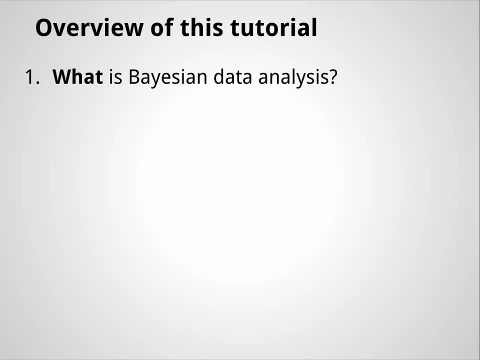 data analysis as one good tool among many that you should have in your data science tool belt. So this tutorial is about the what, the why and how of Bayesian data analysis. Part one, which you are watching right now, tries to answer what is Bayesian data analysis. Part two touches on why you should 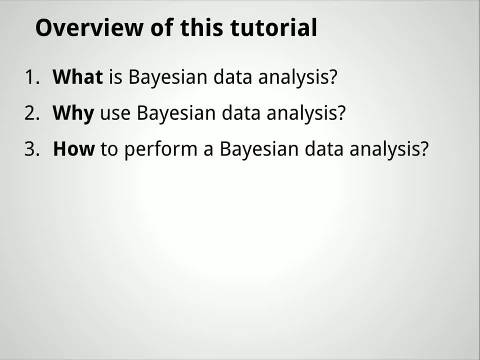 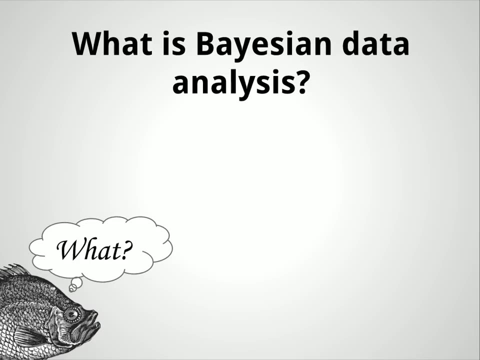 want to use Bayesian data analysis, And part three has some hints on how to actually perform a Bayesian data analysis in practice. So let's start part one proper. What is Bayesian data analysis? Well, this can be characterized in a number of ways, some more helpful than others, One that isn't too helpful but that is correct, is that? 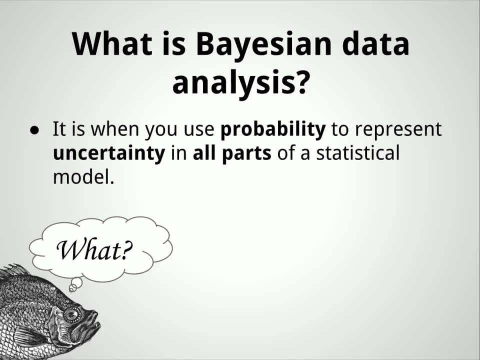 Bayesian statistics is when you use probability to represent uncertainty in all parts of a statistical model. So if you use probability to represent all uncertainty, then you are actually using Bayesian data analysis But, by definition, using a Bayesian model. You could also see Bayesian data analysis. 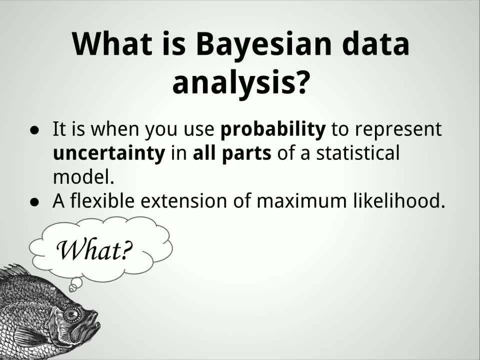 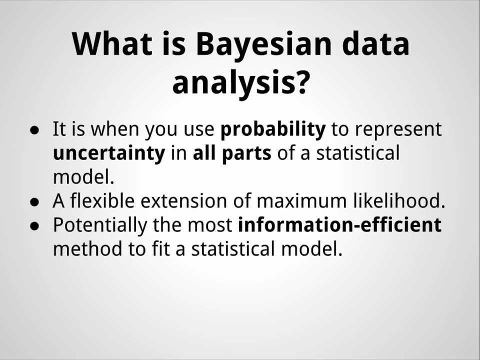 as a flexible extension of maximum likelihood, Maximum likelihood being perhaps the most common way of fitting models in classical statistics. You can also argue that Bayesian data analysis is potentially the most information efficient method to fit a statistical model, But it's also the most computationally intelligent method to fit a statistical model. So if you use Bayesian data, 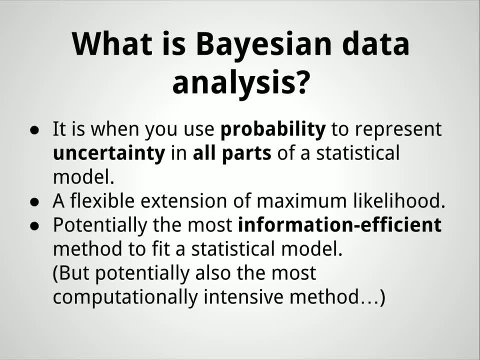 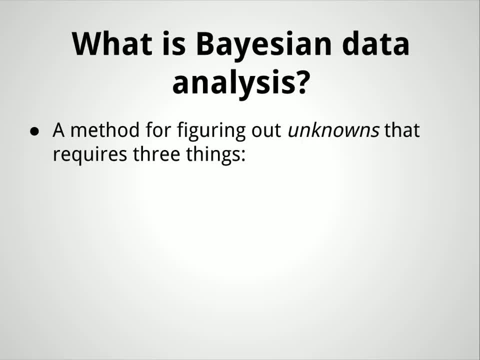 analysis as a flexible extension of maximum likelihood, then you are actually using Bayesian data analysis. The characterization that we're going to run with in this tutorial is the following: Bayesian data analysis is a method for figuring out unknowns, often called parameters. that requires three things: One, data, Two, something. 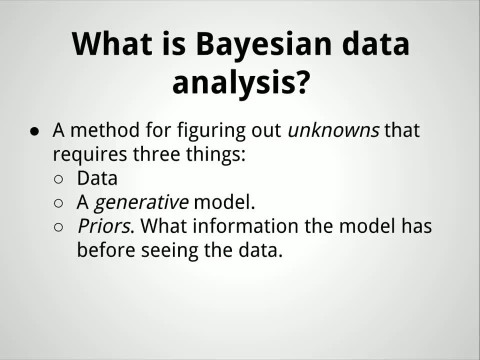 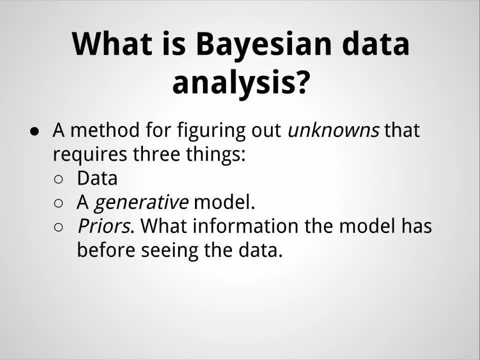 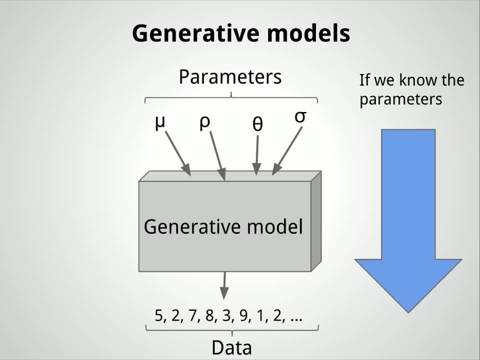 generative model here. Well, it's a very simple concept. It's any kind of computer program or mathematical expression or set of rules that you can feed fixed parameter values and that will generate simulated data. A typical example of a generative model is probability distributions like 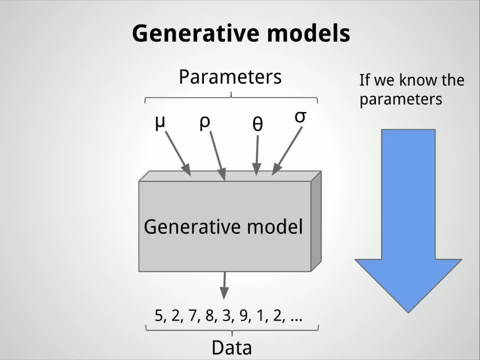 the normal distribution which you can use to simulate data, But also any kind of function that you can whip up in R or Python that simulate data counts as a generative model. So a generative model is great if you know what parameter values you want, but you're interested in how much the data 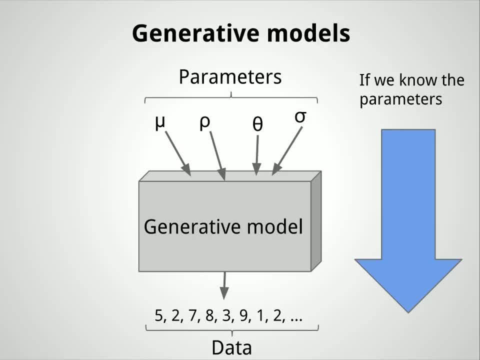 could vary, given those parameters, Because then you can simply plug in those parameter values, run your generative model a large number of times. look at how much the data jumps around. That is, it's a classical Monte Carlo simulation. But often we are in the complete opposite situation. We know what the data is, It's not uncertain And we 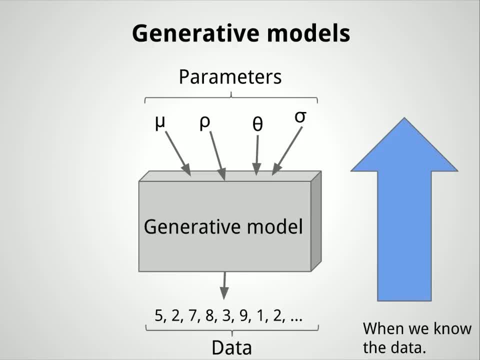 want to know what the data is And we want to know what the data is. And we want to know what the data is And we know what are the reasonable parameter values that could have given rise to this data. That is, we want to work our way. 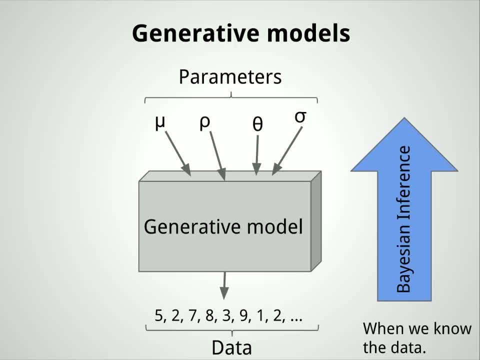 backwards from the data that we know and learn about the parameter values that we don't know. And it is this step the Bayesian inference helps you with. So now I'm going to explain how Bayesian inference works with a motivating example. Well, it's up to you. you if you think it's motivating, but it's about fish, and who doesn't like fish? 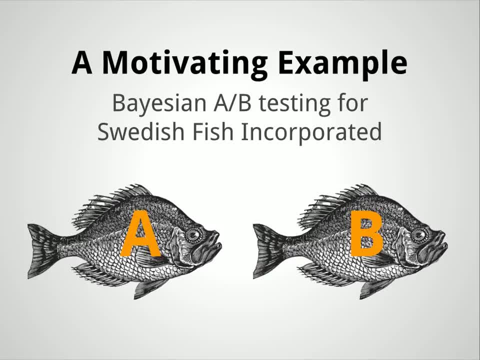 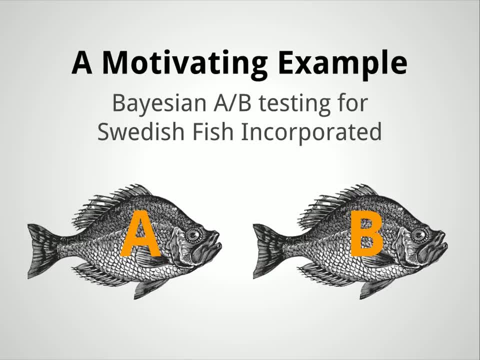 One of the classical uses of inferential statistics. But to keep things simple, we're actually going to start with just estimating the performance of one method, So it's just A-testing, But we'll come around to the B later Now. Swedish Fish Incorporated is a company that makes money by selling fish subscriptions. 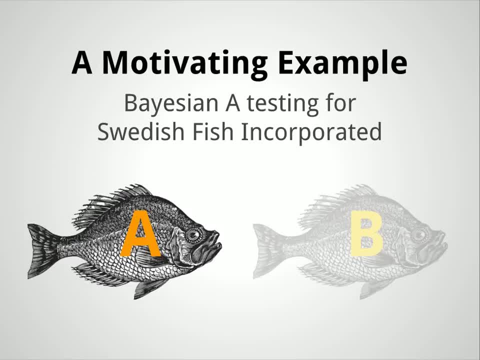 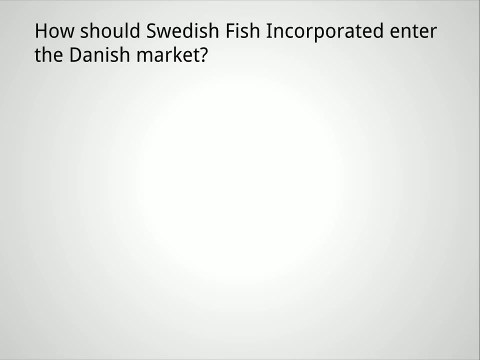 You know, you sign up for a year and every month you get a frozen salmon in the mail. They are huge in Sweden, but now they want to break into the lucrative Danish market. But how should Swedish Fish Incorporated enter the Danish market? Well, the CEO has already come up with a plan. 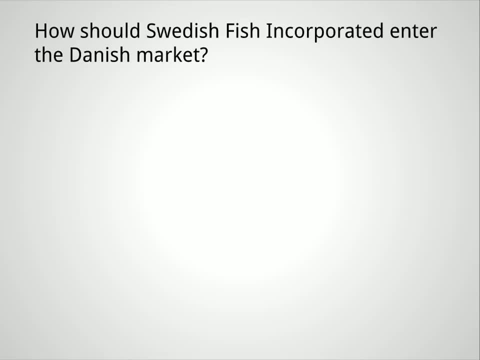 Let's call it methodology, Method A. he put together this colorful brochure which advertises the one-year salmon subscription plan, And marketing has actually already tried this out on 16 randomly chosen Danes, And out of the 16 Danes that got the brochure, six signed up for one year of salmon. 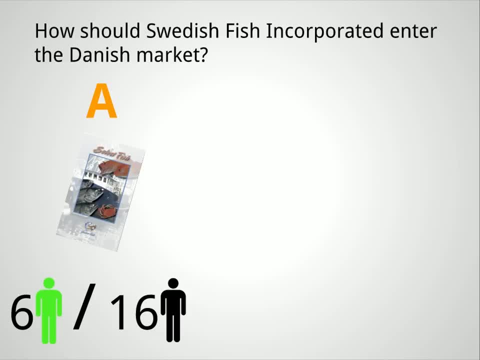 So what we want to know now is: how good is method A? What should we expect the percentage of signups to be If we start sending brochures on a large scale? Well, we could, of course, calculate the percentage of signups in our sample. 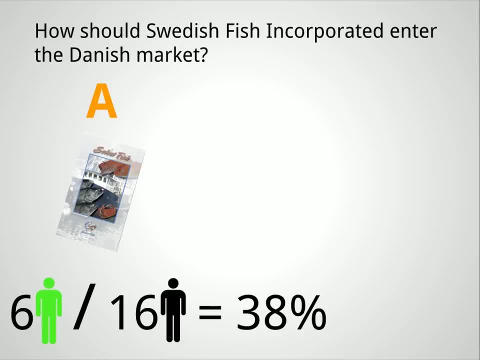 That's just, 6 divided by 16 equals 38 percent, And maybe that is a good guess. but surely this guess is quite uncertain, Especially since we have such a small sample. So not only do we want to know what's a good guess for the percentage of signups, 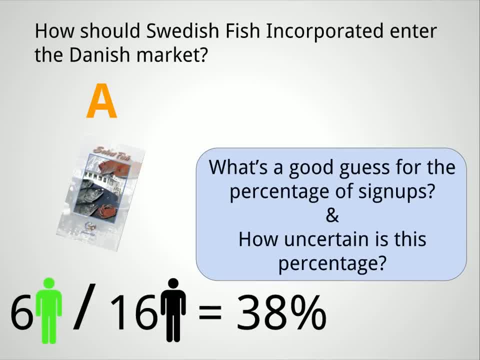 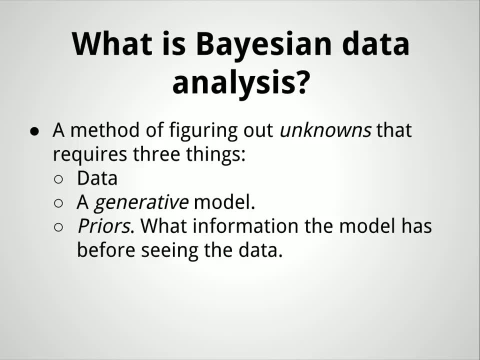 but we also want to know how uncertain is this percentage? And that's what we're going to use Bayesian data analysis for. So remember that Bayesian data analysis requires three things: Data, and we have data, so check on that. Then we need a generative model, which we don't have. 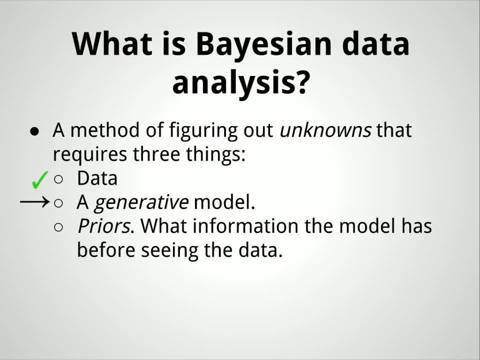 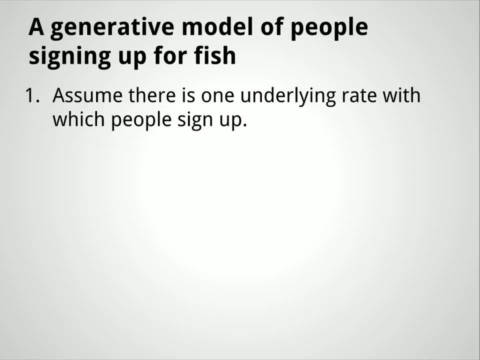 So let's come up with that. Let's come up with a generative model of people signing up for fish. There are, of course, many ways of doing this. I'm just going to go with something simple here. So first, let's assume that there is one underlying rate with which people sign up. 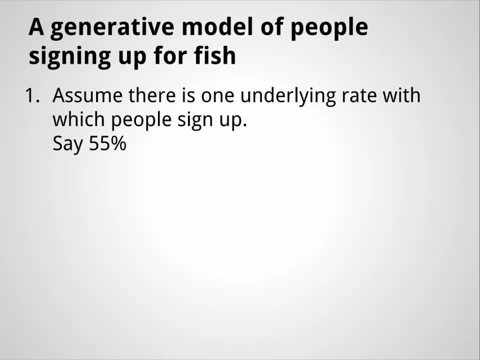 For now let's just have a number, let's say 55 percent. Then we ask a number of people where the chance of each person signing up is then 55 percent. So ask is in quotes here, because we're actually not going to ask anybody. 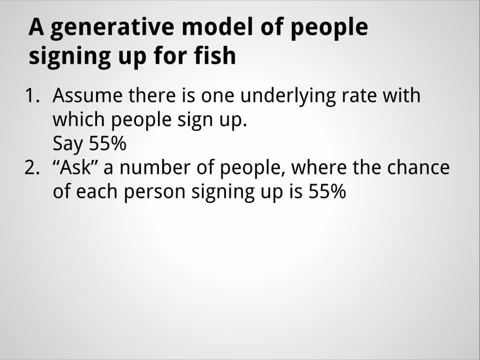 This generative model is something that we could implement in R or Python, And ask And asking here just means we use some random number function where there's a 55 percent chance of getting a yes and a 45 percent chance of getting a no. 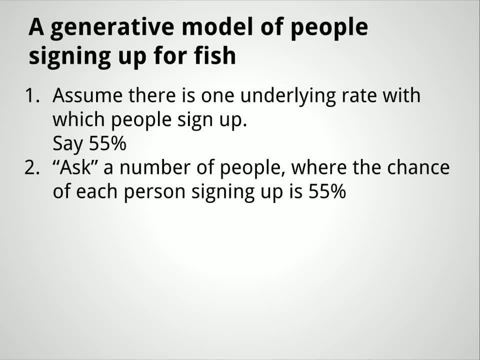 So how could this look? Let's ask in quotes 16 people, because that's how many that was asked in our data set, And let's see how many of those 16 people sign up. So the first person didn't sign up. 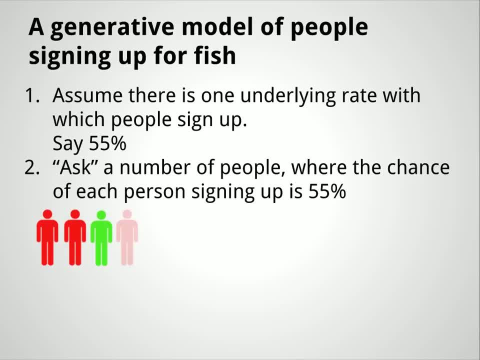 The second person didn't sign up, The third person didn't sign up, The fourth person didn't sign up, The third person signed up, And so on, for all our 16 people, And finally we're going to count how many signed up. 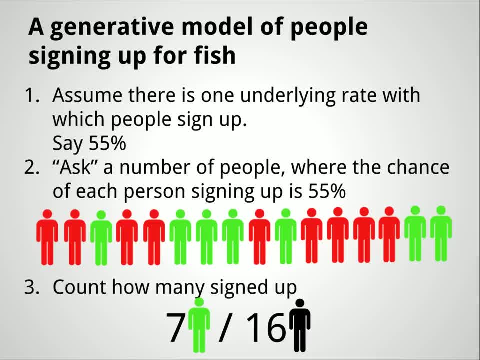 And in this instance, 7 out of 16 people signed up. So this time, 7 out of 16 is our simulated data. Great. So now we have a generative model. We have a model where we can plug in fixed parameter values and generate simulated data. 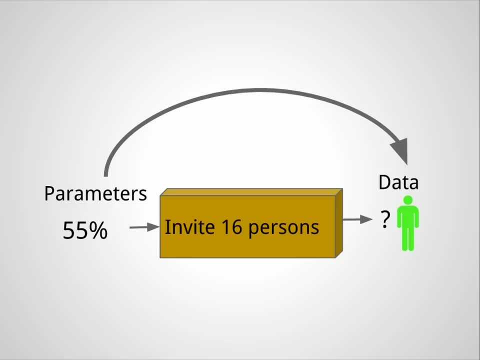 The problem is, of course, that this is the opposite of what we really want. We don't want to simulate data. We know what the data is. We know that when marketing asked 16 randomly selected Danes, 6 of them signed up. 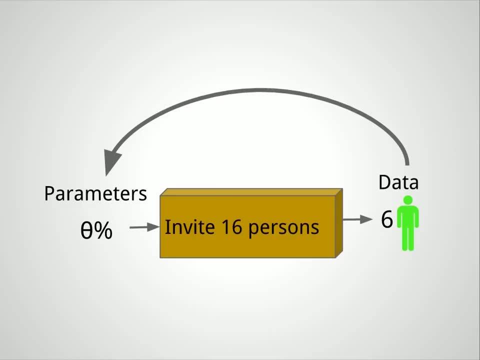 And what we want to do is the opposite. We want to go backwards from the data that we know and figure out what could be reasonable parameters that resulted in this data. That is what is likely, the rate of sign up that resulted in 6 out of 16 signing up. 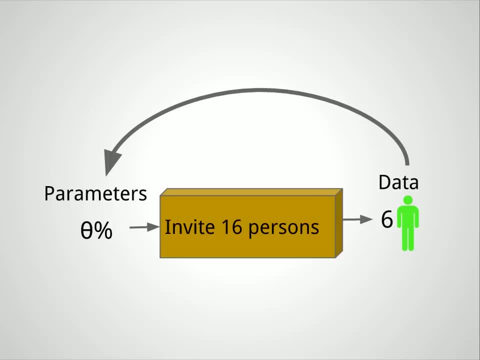 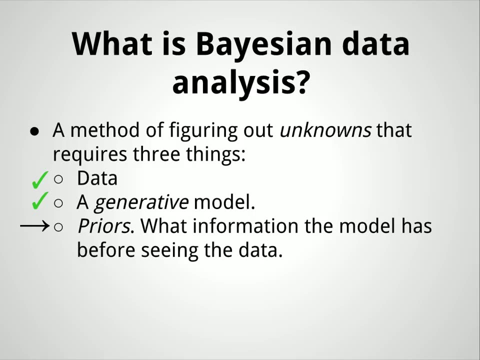 The good news is that we are almost there. We can almost do this. We just need one more thing. We have data, We have a generative model, But we also need priors. We need to specify what information the model has before seeing the data. 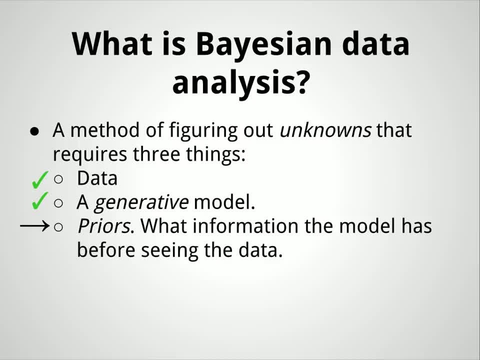 And when you do Bayesian data analysis, that is the same as saying that we need to use probability to represent uncertainty in all parts of the model, And right now we're not doing that. Here is the model We have so far. We have the generative model. 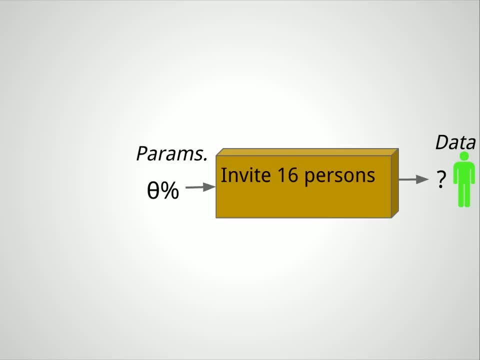 And we have one parameter, one unknown: the overall rate of sign up. If I look at this model, I see uncertainty in two places. There is uncertainty in the generative model. We don't know what the simulated data will be each time we run it. 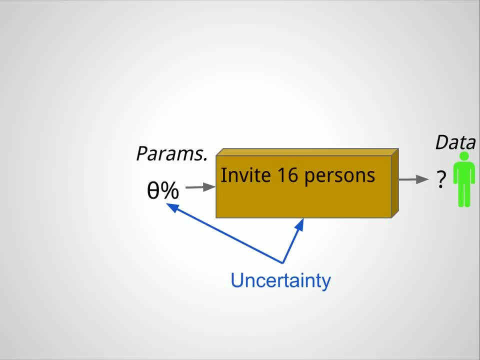 But that uncertainty is already implicitly represented by probability, as we're using a random number function to simulate data And if you know your probability distributions, you might have already recognized that the generative model is actually the same as a binomial probability distribution. But there is also uncertainty in what the parameter value is. 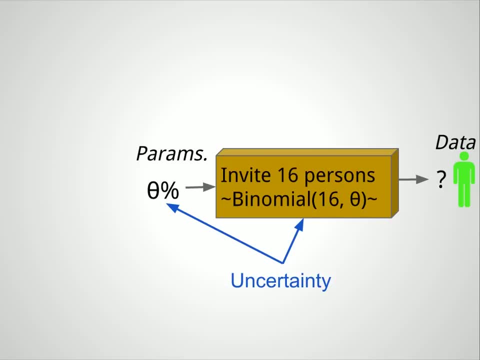 the overall rate of sign up, And that uncertainty is yet not represented by any probability or probability distribution. So let's do that. There are many different ways you could go about this, But I'm just going to use an easy, off-the-shelf solution. 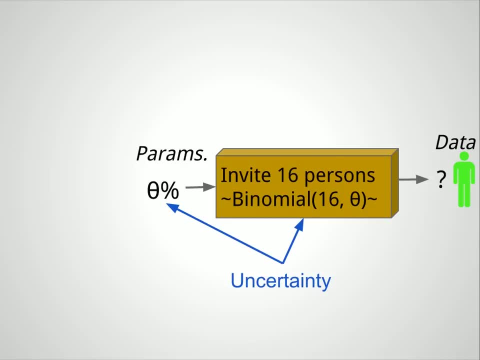 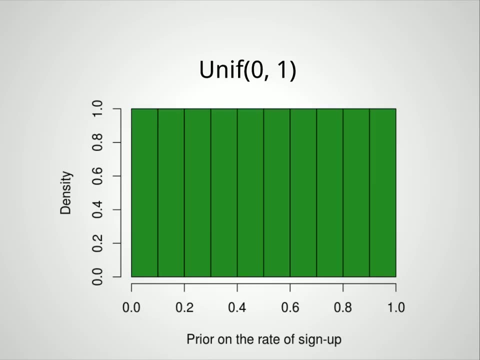 I'm going to represent the uncertainty regarding the overall rate of sign up by a uniform probability distribution from 0 to 1.. That is, by using this probability distribution, we're stating that, prior to seeing any data, the model assumes that any rate of sign up between 0 and 1 is equally likely. 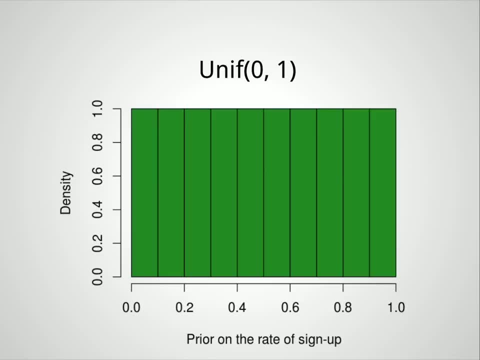 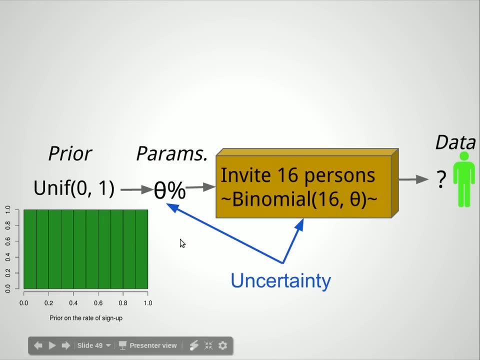 The probability distributions that are used in this way to represent what the model knows prior to seeing the data are called often prior distributions or just priors. All right, so now we have specified the prior and all uncertainty in the model is represented by probability. 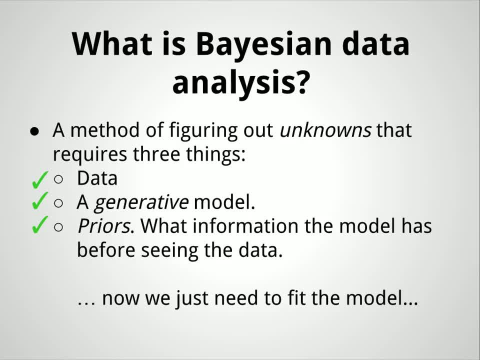 If we now look at our checklist, we see that we have data, a generative model and priors, and we should be ready to roll. Now we just need to fit the model somehow. Again, there are many different ways of doing this. 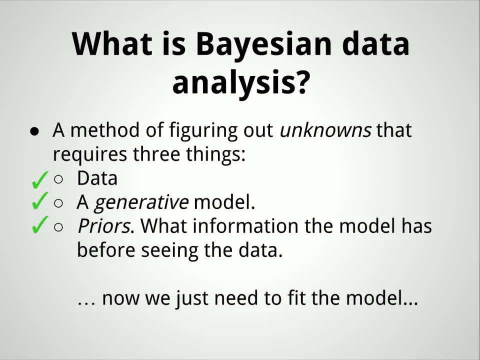 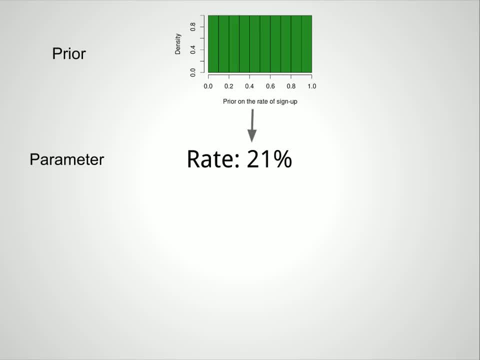 but here is one that is conceptually simple. First, we're going to start with our prior And we're going to draw a random parameter value from it. This time it happened to be 0.21.. That is a rate of sign up of 21%. 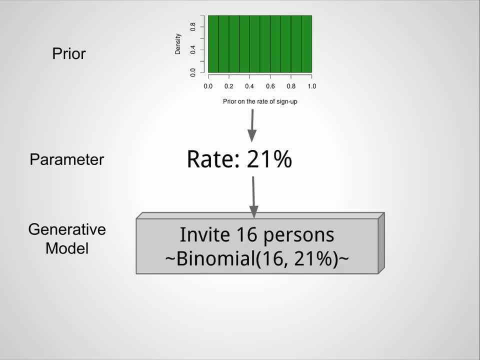 Then we're going to take this parameter, draw and plug it into our generative model And we're going to use it to simulate some data. This time, when we ran our generative model, 4 out of 16 signed up for a year of Salmon. 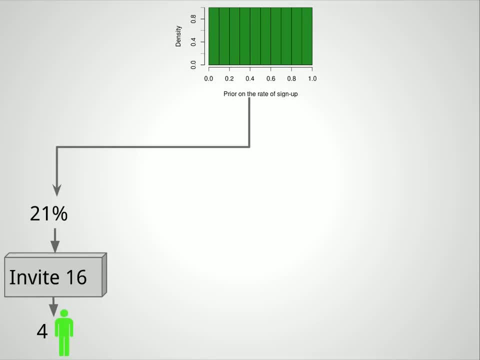 And now we're going to do what we just did: drawing from the prior And simulating data many, many times, Say 100,000 times. So we're drawing from the prior and simulating data Again And again. 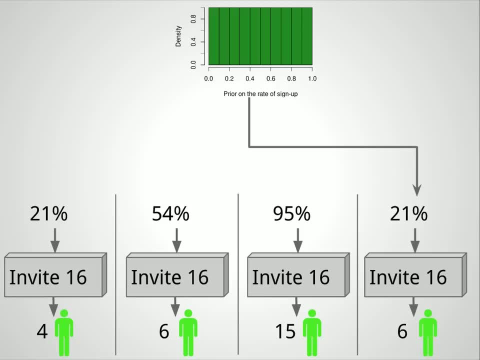 100,000 times, But here we're just looking at the first four, But really 100,000 times. Now it's time to bring in what we actually know. Now it's time to bring in the data, Because if it is something we know, 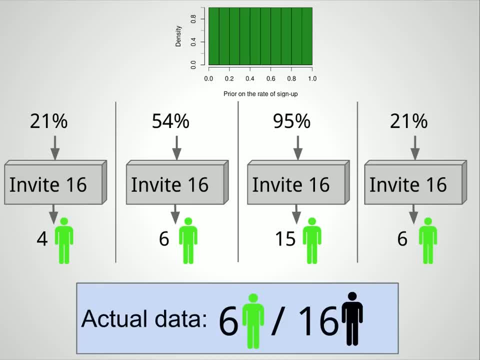 it is that when marketing did this for real, 6 out of 16, people signed up. So now we're going to filter away all those parameter draws that didn't result in data consistent with what we actually observed. That's because we're interested in reality. 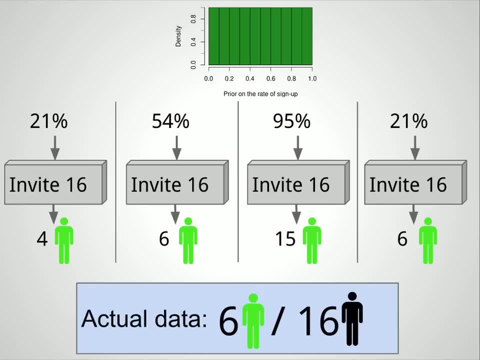 And what a reasonable rate of sign up could be in reality. And in reality, 6 out of 16 people signed up. So we're going to remove the first parameter draw because it didn't result in 6 people signing up. We're going to keep the second as the parameter draw. 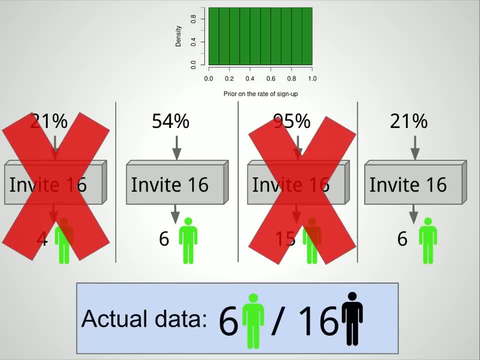 actually resulted in 6 people signing up. We're removing the third And we're keeping the fourth, because it resulted in 6 people signing up And so on for all the 100,000 parameter draws. Note that sometimes we keep a certain parameter value. 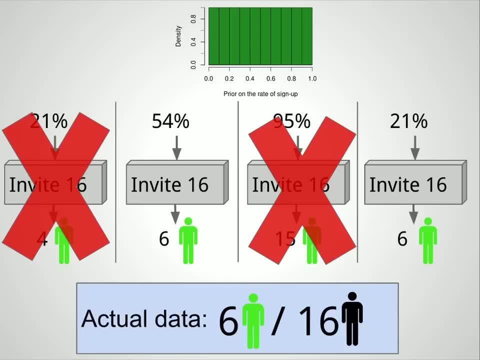 and sometimes we filter the very same value away. It all depends on whether the generative model simulated matching data that specific time. So, for example, here we toss the first 21% parameter draw, but we're keeping the fourth. So what did all this work give us? 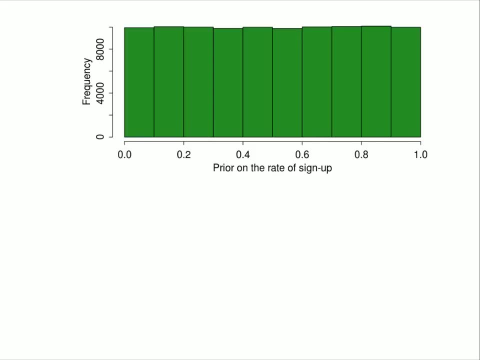 Well, this is what we saw. This is what we started with. This is the distribution of the 100,000 draws from the prior before we did the filtering step. As the prior was a uniform distribution between 0 and 1,, you shouldn't be too surprised to see that the 100,000 random draws 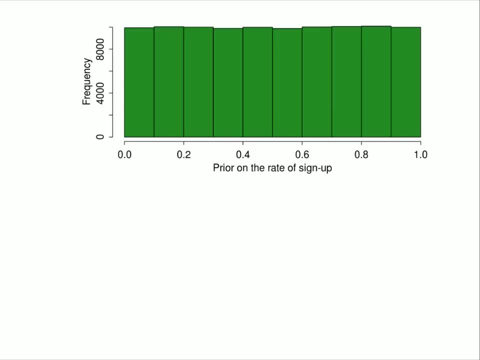 form a pretty uniform distribution, But if you look carefully you see that the bars actually are slightly different. Then, after having done the filtering step, where we removed all the parameter draws that didn't result in matching data, that's the distribution we ended up with. 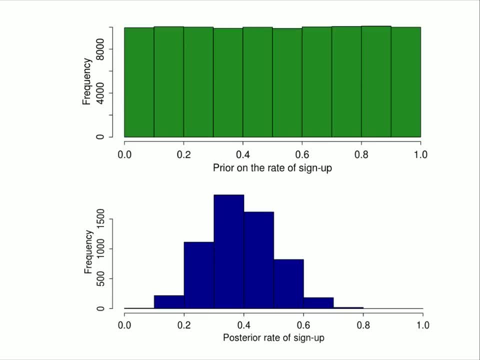 And this blue post-filtering distribution is actually the answer to our original question about what a likely value of the sign-up rate is, Because a parameter value that is more likely to generate the data that we collected is going to be proportionally more common in this blue distribution. 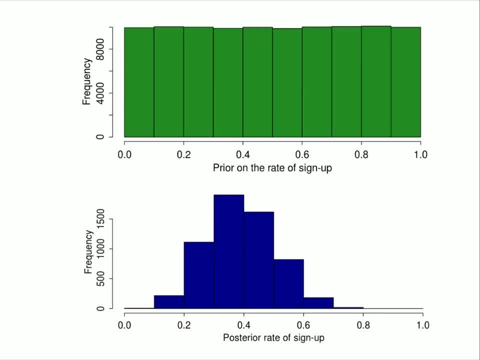 That is a parameter value that is twice as likely as some other parameter value to generate the data we actually saw is roughly going to be twice as likely, going to be twice as likely as some other parameter value to generate the data we actually saw as common in this blue distribution. So right away we can see just by looking at the distribution. 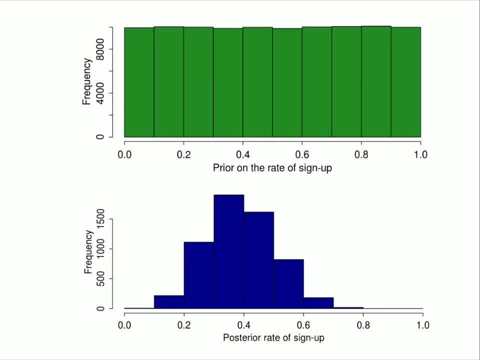 that parameter values below 0.1 and above 0.8 almost never resulted in the data we observed, So it should be very unlikely that the signup rate for Salmon's subscription is below 10% or above 80%. We see that the subscription rate is likely somewhere between 20% and 60%. 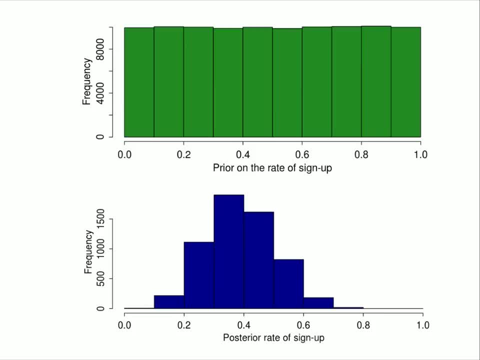 with it most likely being between 30% and 40%, But, importantly, we see that the distribution is pretty wide, which means that, even after using our not-so-impressive data set of 16 data points, the signup rate is still very uncertain, And Bayesian data analysis was all about representing. 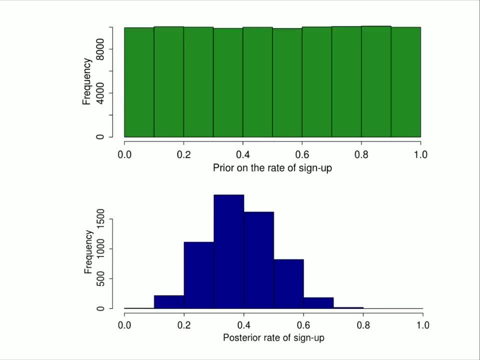 uncertainty with probability, but we still haven't calculated any probabilities. but since we have a distribution of samples, it's easy to do. Say that we want to calculate the probability that the signup rate is between 30% and 40%. say Then we first count up how many. 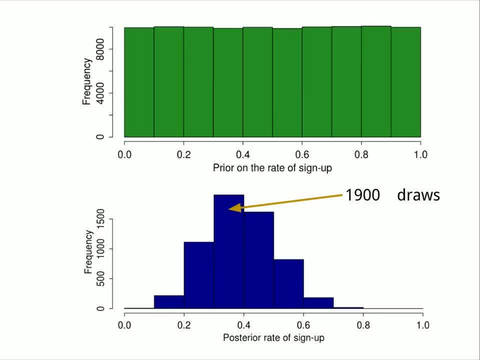 parameter draws that are between 0.3 and 0.4.. Here it was 1,900.. And then we divide by the total number of draws that survived the filtering step, which was 5,700.. And if we divide 1,900 by: 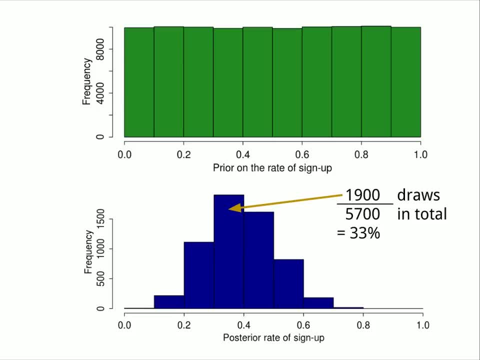 5,700, we get that there is a 33% probability that the signup rate is between 30% and 40%. We can, of course, do the same calculation for all the bars of the distribution, And what we end up with is a probability distribution over likely signup rates. 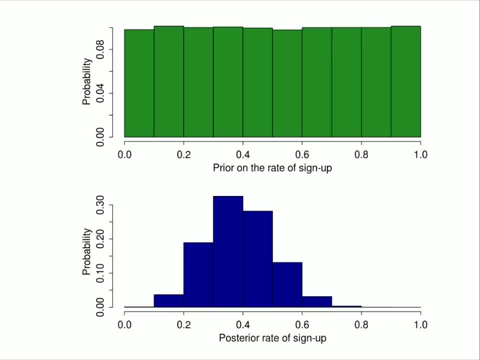 Now it's important to note that this probability distribution doesn't stand on its own. It's always given the assumptions and the data we used. In Bayesian jargon, these two distributions are called the prior and the posterior distribution. That's because the prior distribution is what the 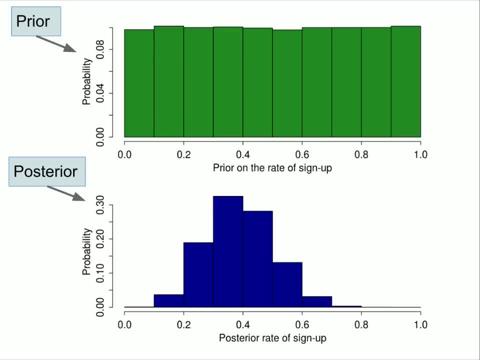 model knows about. the parameter And the posterior distribution is what the model knows about. the parameters before, prior to using the information in the data, And the posterior distribution is what the model knows about the parameters after, posterior to having used the data in the filtering. 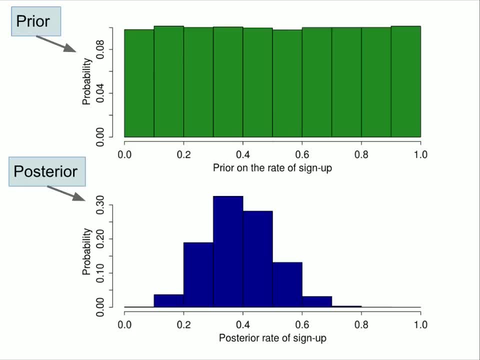 step Now. the posterior distribution is really the end product of a Bayesian analysis. It contains both the information from the model and from the data, And we can use it to answer all kinds of questions. For example, what signup rate is the most probable? 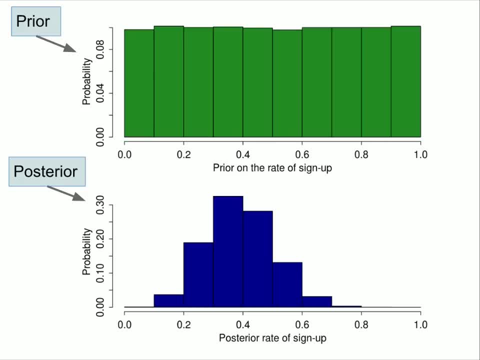 This is just the parameter value with the highest probability in the posterior. Since the plot of the posterior is binned into 10% spins, it's a little difficult to read from the plot, But the signup rate with the highest probability is actually 38%. So if we just had to report a 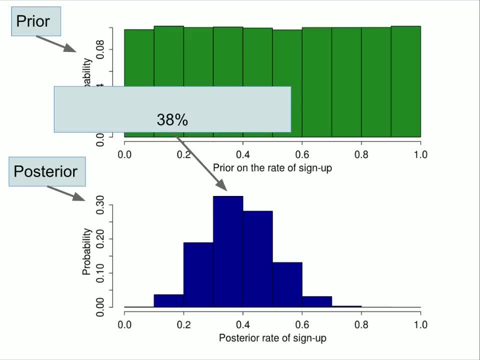 single number, 38%, could be given as a best guess. Now, as we used uniform prior, this is actually also the parameter value that is the most likely to be the highest probability. So if we just had to generate the data we actually observed- And in classical statistics this type of estimate is- 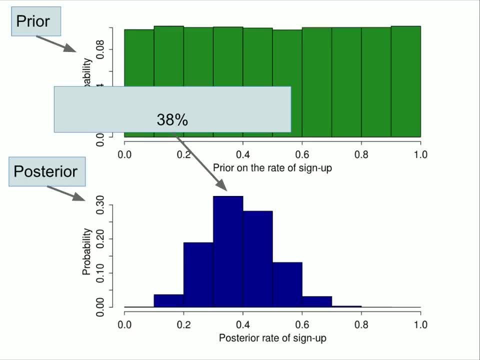 well known under a specific name. Do you want to guess? It's the parameter value with the maximum likelihood to generate the data we observed. Yeah, it's the so-called maximum likelihood estimate, And maximum likelihood estimation is one of the most common ways of fitting models in classical 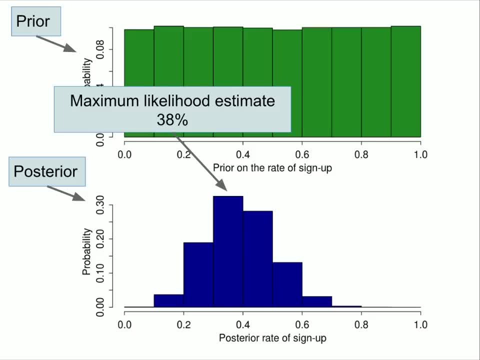 statistics, And this is the reason for why Bayesian data analysis can be seen as a extension of maximum likelihood estimation, Because as long as you use flat priors, you'll always get the maximum likelihood estimate for free when you fit a Bayesian model. But there 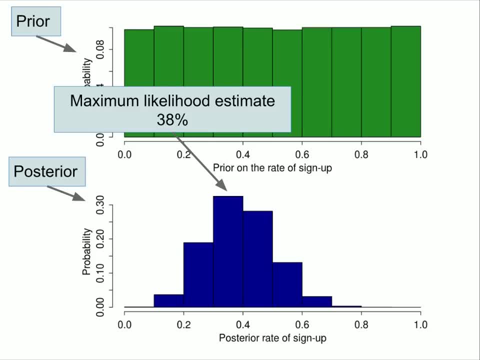 are other ways you can summarize a posterior distribution except for the maximum likelihood estimate. You can take the mean of the posterior distribution, the posterior mean, as another best guess of the rate of signup. In this case it's almost the same as the maximum likelihood estimate. 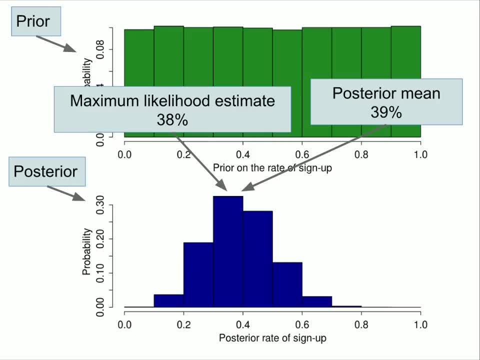 but that's not always the case. Or you might want to summarize the uncertainty of the signup rate as an interval, And then you can find the shortest interval that covers, say, 90% of the probability. This is often called a credible interval, And here 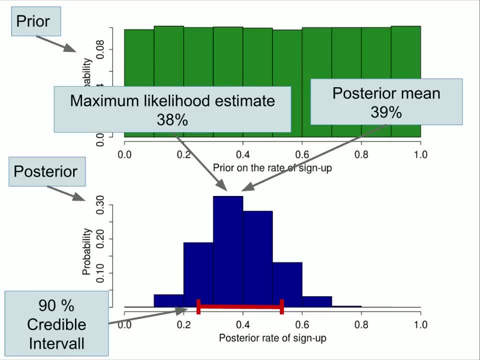 we can see that the 90% credible interval go between 0.3 and 0.54.. So we can state that the signup rate is between 30 and 54%, with 90% probability. All right, that was a simple example of Bayesian data analysis, And at this point in the tutorial we usually do a small. 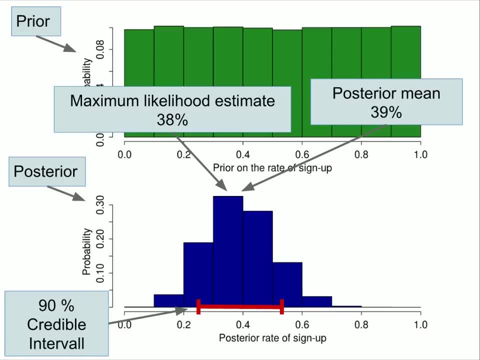 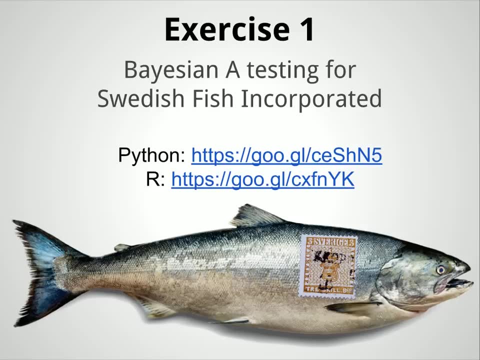 exercise where we replicate the analysis I just described to you. So if you are in front of a computer and have either R or Python installed, I recommend that you pause this video and try out this exercise by following either of the links here. It's a really useful exercise for helping. 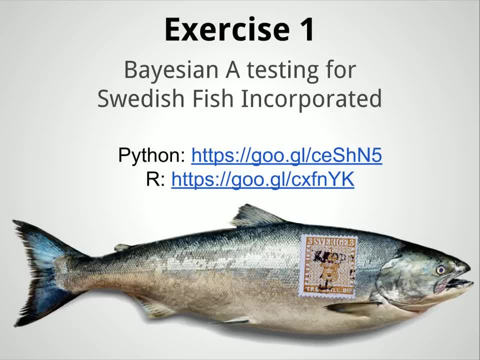 you understand Bayesian data analysis, So pause. pause the video now and do it. I'll be waiting for you when you come back. All right, okay, Welcome back. I hope the exercise went well And if it didn't, you should take a look. 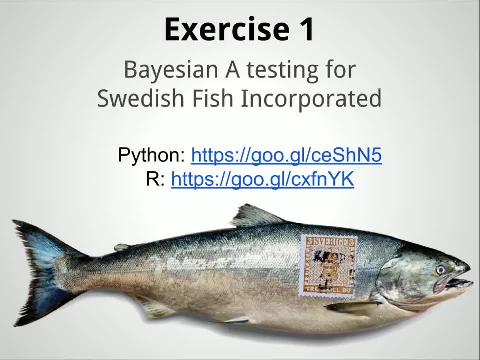 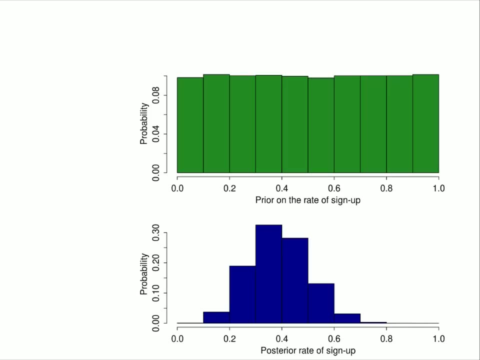 at the solution at the bottom of the exercise page. Now we're going to go through what we just did, So nothing new. But this time we're going to use a tiny bit of math notation. So the green distribution here is the prior, That's what we started with, And the blue distribution is the posterior, That's what. 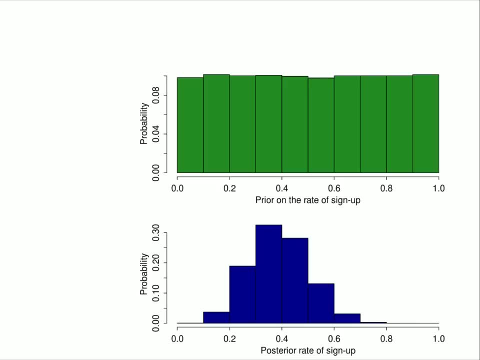 we ended up with after having used the data. So how did we go from the prior to the posterior? Let's take a signup rate of 35% as an example. First, a signup rate of 35% had to be drawn from the prior. 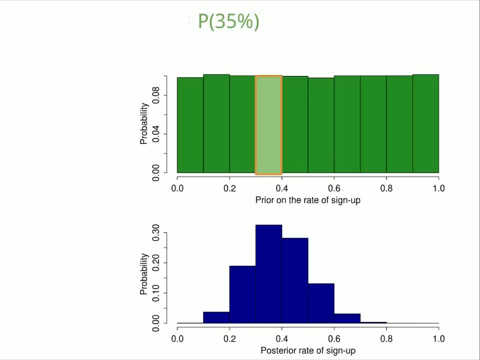 And that it did with some probability. Here the P with parentheses stand for the probability of drawing a parameter value of 35% from the prior. Then, in order to not throw this parameter draw away, it had to simulate data which matched the data we actually observed, And that it also did. 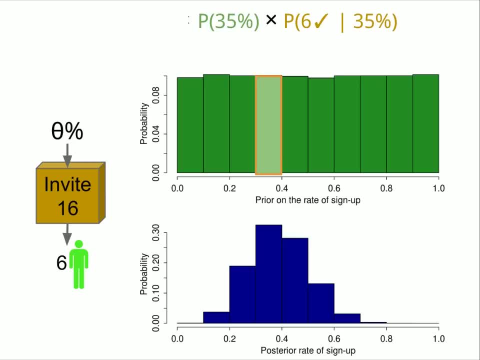 with some probability Here, the P with the vertical bar stands for the probability of generating six signups. given The bar should be read as: given A parameter value of 35%, And by multiplying these two probabilities together we get the probability of first generating a signup rate of 35% and then simulating data. 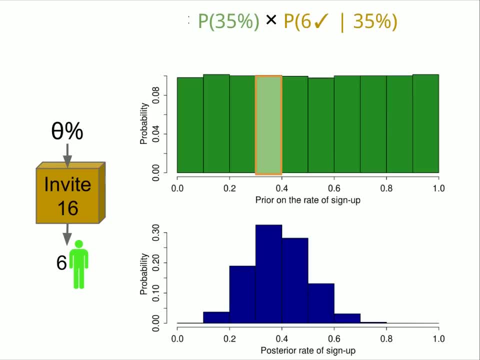 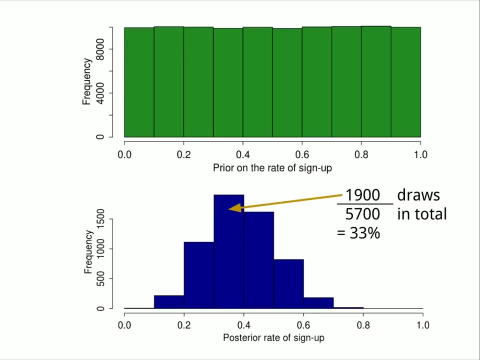 that matched the data we observed, And this will be proportional to the probability of 35% being the best parameter value given the data. This is in the same way as before, where the P was proportional to the probability of the signup rate being in that range. 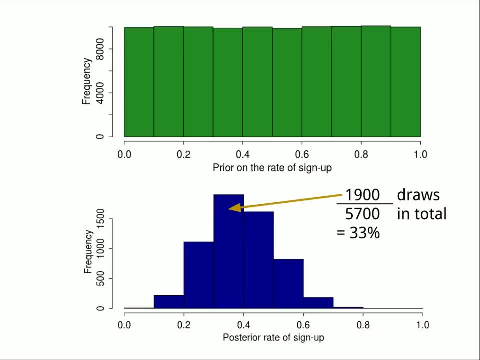 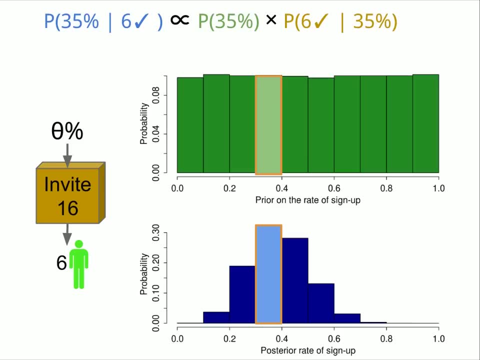 But it wasn't a probability. It was 1900 parameter draws. So it wasn't a probability until we, divided by the total number of draws, And in the same way we have to here divide by the total sum of the probabilities of generating the data for all the parameter values, And this gives us the probability of 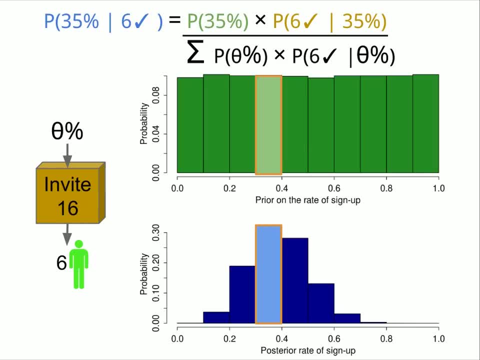 a signup rate of 35%, given the data. And, of course, we could use the same procedure for all the other signup rates to retrieve a full probability distribution. Again, this was nothing new. This is just what we did before, but now using a little bit of probability notation. So what have we done? We have specified prior. 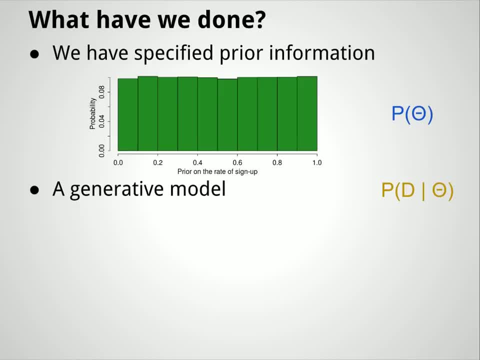 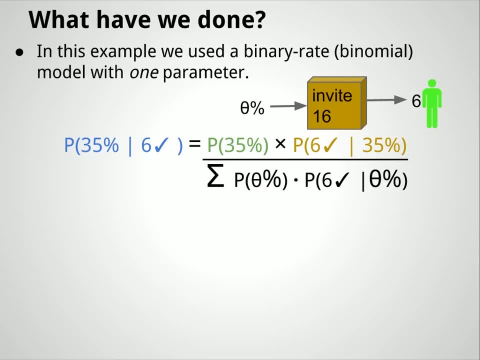 information And we have calculated the probability of different parameter values given the data. In this example, we used a binary rate binomial model with one parameter, But the cool thing here is that the general method works for any generative model with any number of parameters, That is. 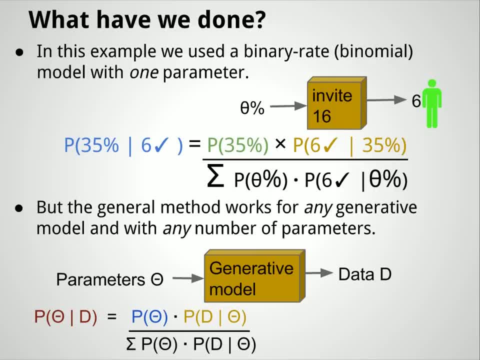 you can have any number of unknowns, also known as parameters, that you plug into any generative model that you can implement, And the data can be multivariate or it can consist of completely different data sets, And the Bayesian machinery that we used in the simple case works in the 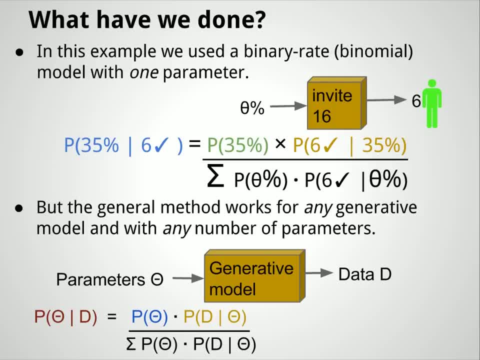 same way here. Now the equation down at the bottom here is just a generalized version of the one we used in the Salmon subscription problem, where here, d is the data and the theta, the o with the dash through, are the parameters. So this equation isn't anything new, It's just what we did before, And that equation is what's. 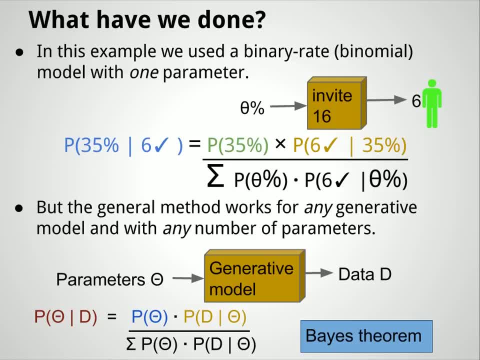 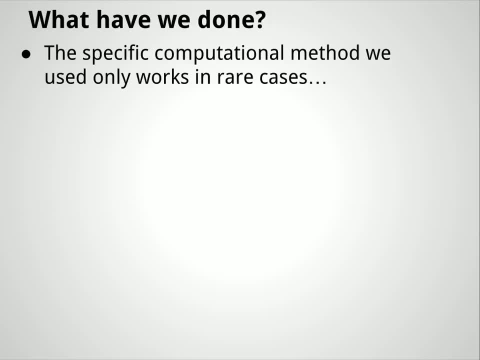 usually called Bayes' Theorem. So there it is. Now I need to mention that the specific computational method we used in the Salmon subscription problem only work in rare cases. It's called approximate Bayesian computation, And what's specific to this method is that you code up a generative model, then simulate from it and only 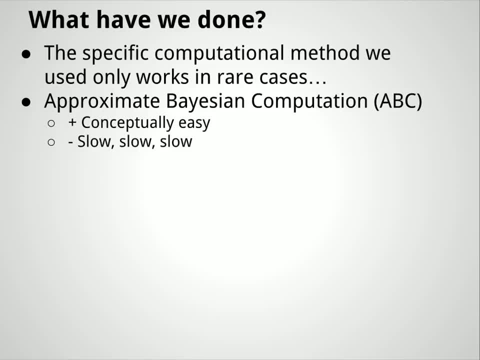 keep parameter draws that match the data, And it's a good method because it's conceptually simple. And it's a good method because it's conceptually simple. But it's a bad method because it can be incredibly slow and scales horribly with larger data if used naively. 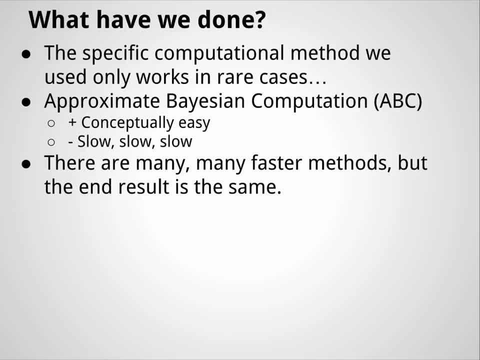 But there are many, many faster methods that are faster because they can take computational shortcuts. But the important part is that if one of those faster methods worked, the end result will be the same as if you would have used approximate Bayesian computation. You will just get the answer much, much faster. 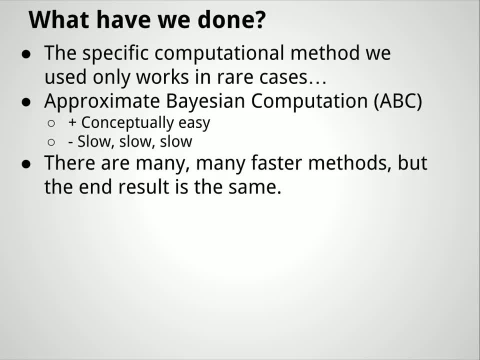 So if you hear about a cool method like Hamiltonian Monte Carlo, you don't need to be too nervous if you don't know how it works, because it's just another method of fitting Bayesian models And when it works the output will be the same as if you would have fitted the model using approximate Bayesian computation. 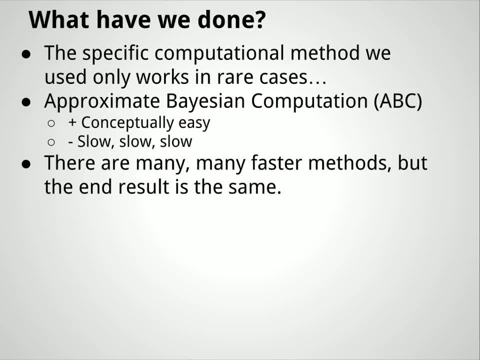 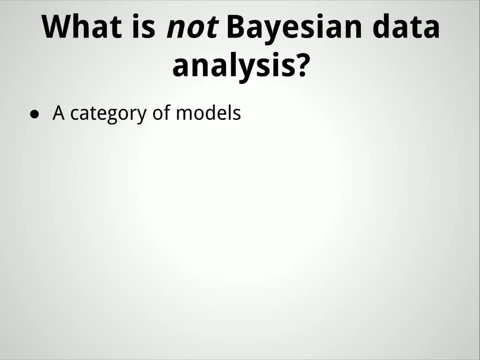 But Hamiltonian Monte Carlo will probably get you the result today rather than in a hundred years, say So now we talked about what Bayesian data analysis is. Let's talk a little bit about what it is not. So first, it's not a category of models. 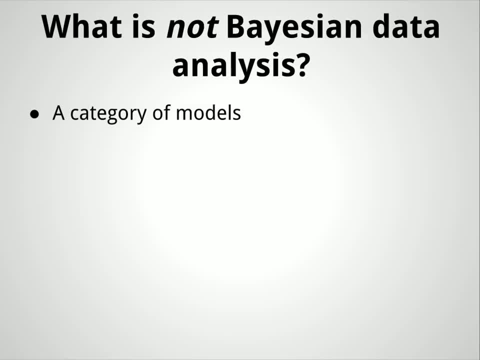 It's not like you have regression models, decision trees, neural networks and Bayesian models. Bayesian data analysis is more a way of thinking about and constructing models, And many parts of statistics and machine learning can be done in a Bayesian framework. So you can have Bayesian regression models, Bayesian decision trees, Bayesian neural networks and Bayesian data analysis. 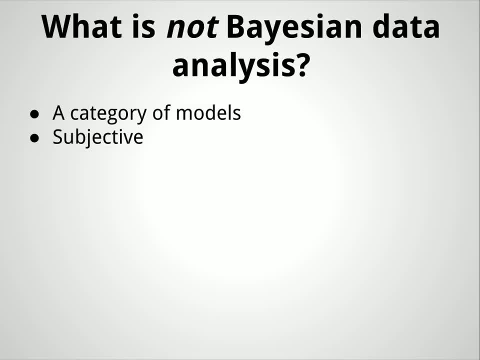 neural networks and so on. Bayesian data analysis is also not more subjective than other types of statistics, as far as I can see, or rather, all statistics is equally subjective. All statistical methods require that you make some assumptions, and the result always has to. 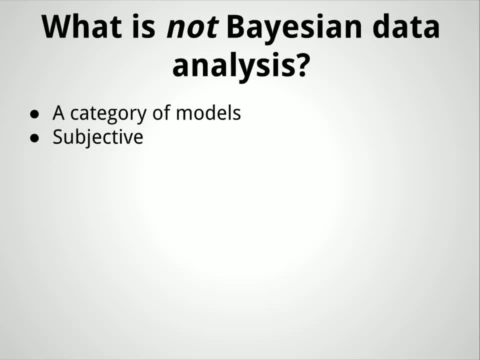 be interpreted in the light of those assumptions. It's the same in Bayesian statistics and in classical statistics Also, even though Bayesian methods has become more popular quite recently, starting in the 90s, when suddenly everybody got the PC. it's important to remember that it is. 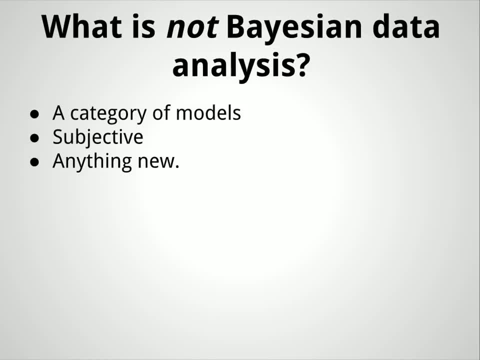 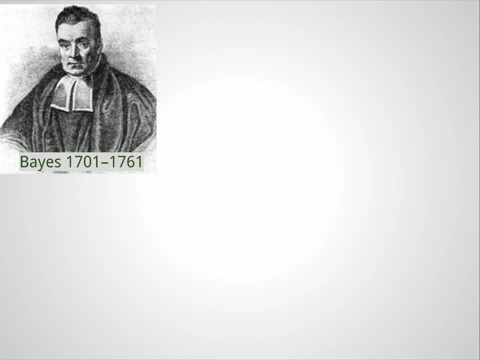 not anything new. It's actually called Bayesian because of this guy, Thomas Bayes, who lived in the 1700s. It's named after him because he failed to publish an essay on solving a specific probability problem, but which was then published after his death. But Bayesian statistics should. 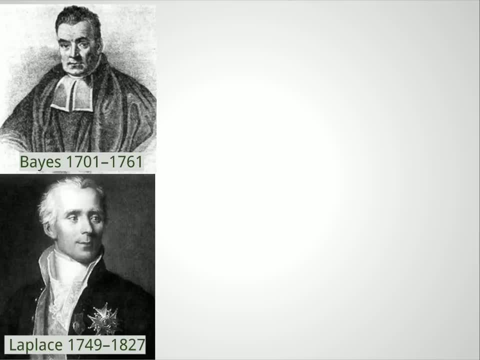 really be named after this guy, This guy, Pierre-Simon Laplace, who was first to describe the general theory of Bayesian data analysis. But he didn't call it Bayesian, rather he called it inverse probability, which sort of makes sense, as you use probability to reversely go backwards from what we know, the data to figure. 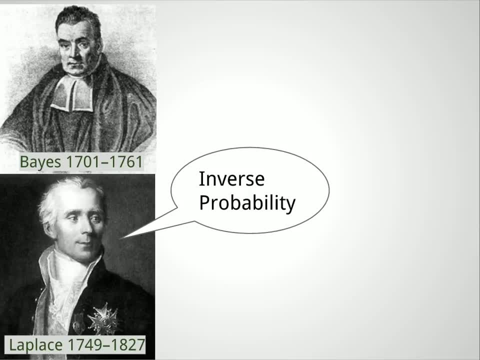 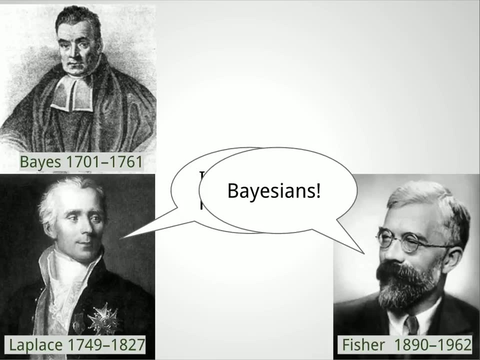 out what we don't know, the parameters. The first known person to have used the word Bayesian was actually Ronald Fisher, the guy that popularized the P-type of data analysis, And he didn't meant it as a compliment, because he famously loathed Bayesian statistics. 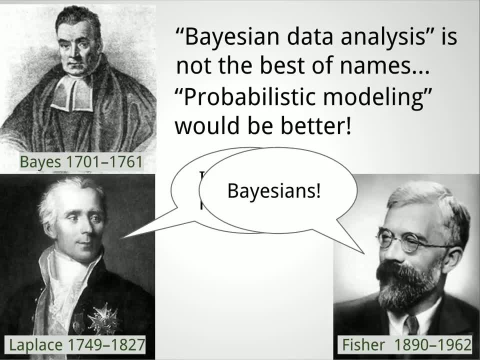 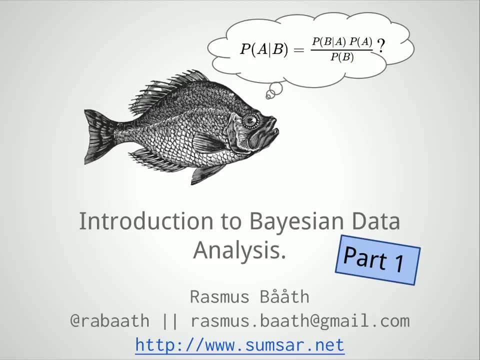 So maybe Bayesian data analysis is not the best of names, and a better name would actually just be probabilistic modeling, because that's really just what it is. Alright, that concludes part one of this three-part introduction to Bayesian data analysis. Now that we know what Bayesian data analysis is,